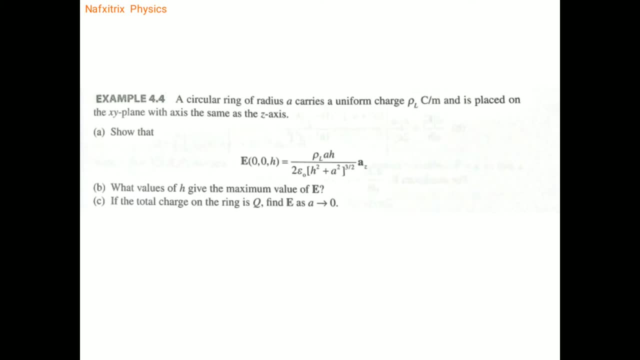 that. So here is the question, Not only electric field, some other points also. So here a circular ring of radius A carries a uniform charge, rho L coulomb per meter. So here we need to consider a circular ring. So it is a ring and it is of radius A, So its radius 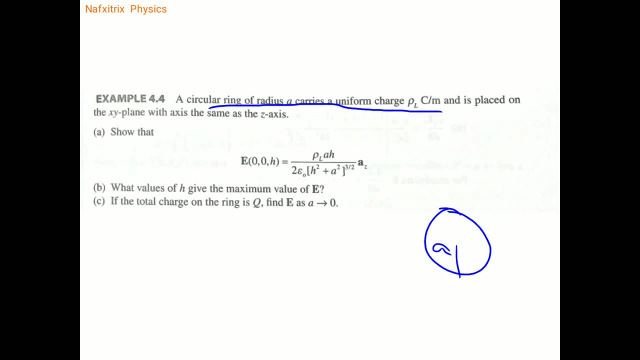 is A of uniform charge. That is, the entire ring is having charge density, So it is a charge density of uniform charge. rho L coulomb per meter, That means charge for unit length. So that is nothing but rho L and is placed on the x- y plane with the axis same as the. 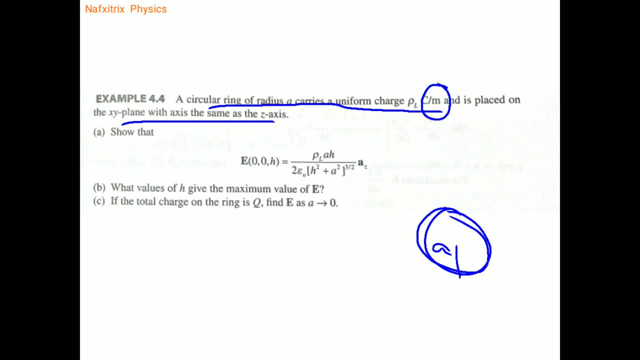 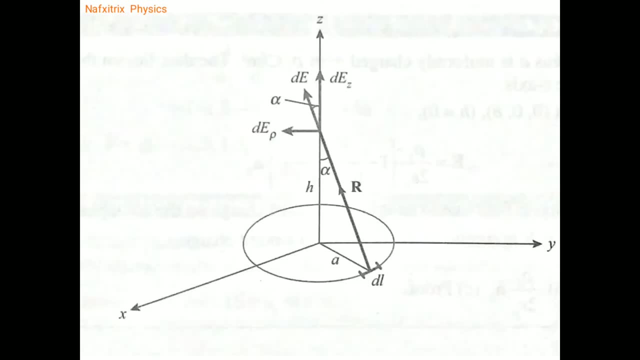 z axis. So this ring is placed in x y plane with axis as the z axis. So best diagram is this. So here it is. So you can see, this is x axis, this is y axis, So the ring is lying in this plane. 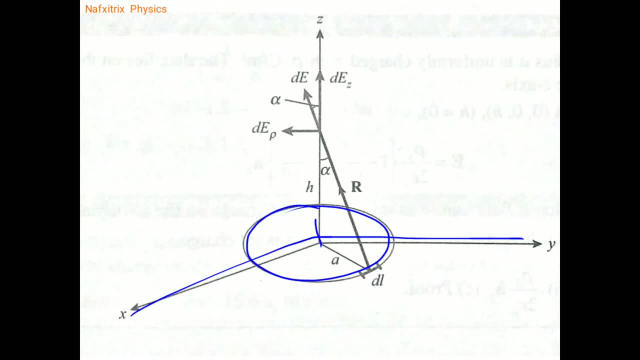 So it is lying in this x- y plane and this is z axis perpendicular to this. So its axis is in the direction of z. So it is lying in this x y plane, perpendicular to this. So this is the arrangement, actual arrangement. So we need to show that E of 0, 0, H is the. 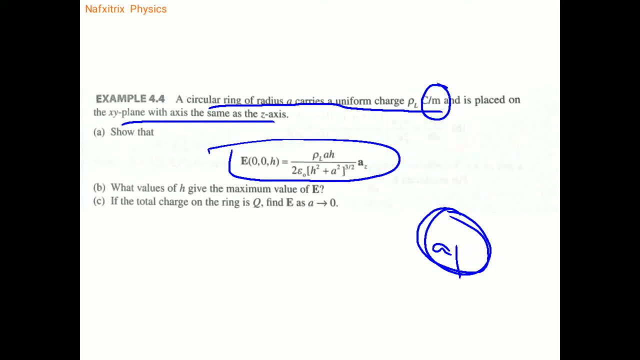 opposite of H. So this one we need to show electric field at certain height. and next point b is values of H, given the maximum value of E. So for what value of H? Q is the maximum value of E, So that one we need to see Total charge on the ring is Q Find E. So if the 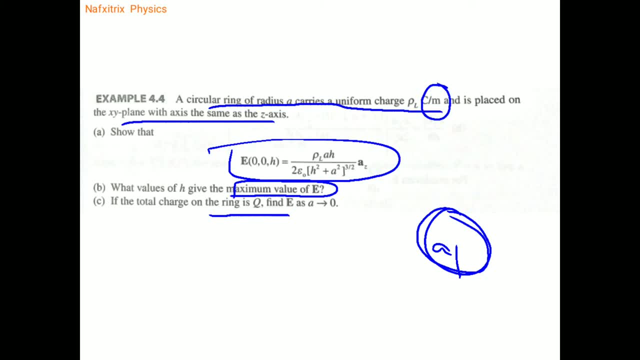 total charge on that ring is Q, we need to find E, as A tends to 0, as A tends to 0. So we need to find E. So if the total charge on the ring is Q, we need to find E, So we. 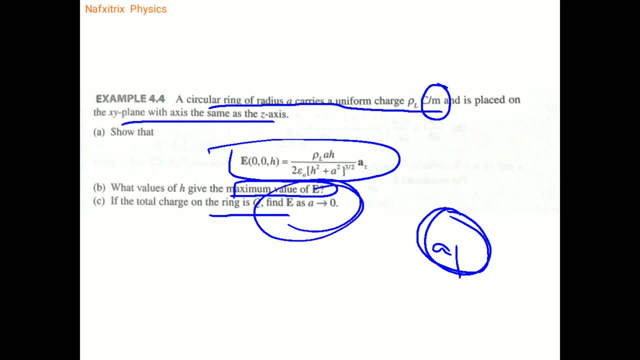 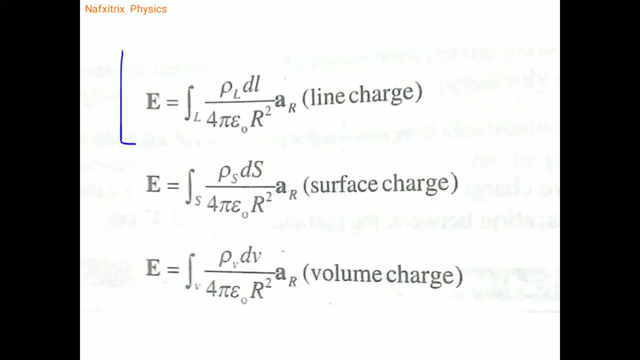 to 0, we need to find e. so this is the question. so for this we need to use this formula here. so this royal is nothing but charge per unit length. that is charge per unit length. that is nothing but lambda. actually we used to indicate it with lambda, but here it is given as royal. 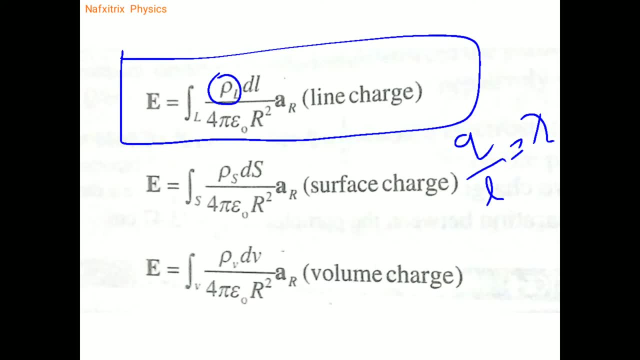 so integration of. actually we know that electric field is nothing but 1 by 4 pi, epsilon naught into q by r square. so it is into q by r square. so this is the formula for electric field. so here, 1 by 4 pi, epsilon naught r square. everything as usual. q is nothing but. 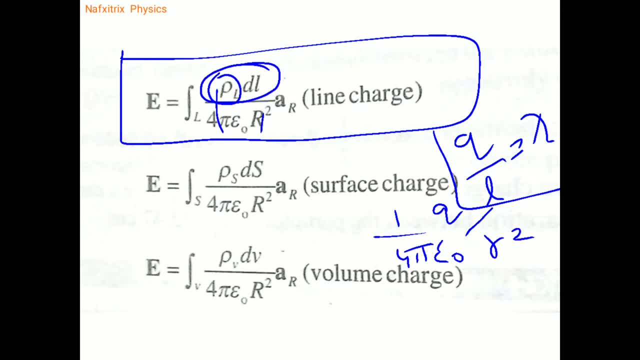 dou l into dl, royal into dl. so in the place of instead of indicating with lambda here, it is given as rho l. that means length charge density, that is, and surface charge density, that is actually sigma. but it is given as rho s, that is nothing but charge per unit area. so this is for 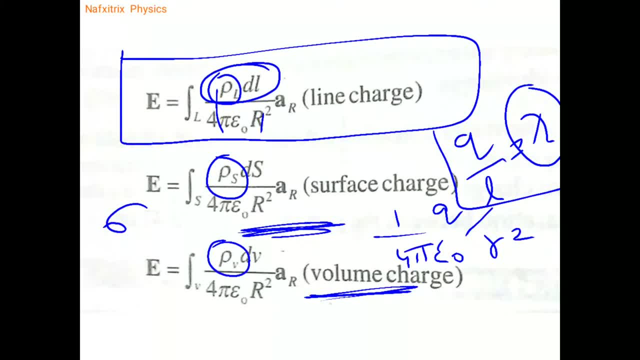 surface charge and this is for the volume charge. so here it is indicated as rho v instead of rho. so that's so here, instead of lambda, royal is nothing but equal to lambda. so notations have been different here. so we need to use this formula. so that is, in the place of q we are having this. 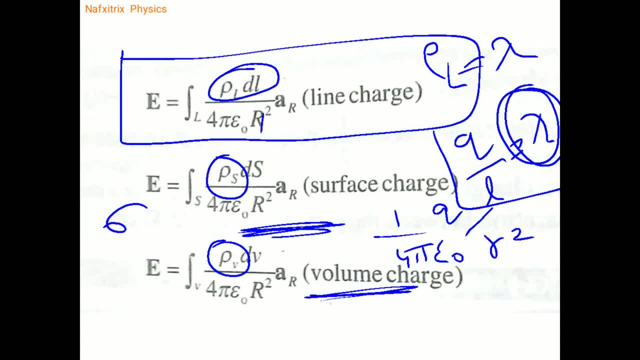 is nothing but q lamb royal into dl charge for a certain length of the thing, small unit length of the ring. so if we do integration for the entire length we would get the electric field. so q by 4 pi. epsilon naught r square and this is unit vector. so it is just a cap, just like r by magnitude of. 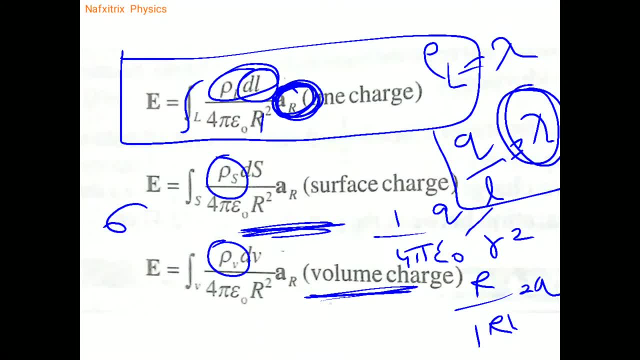 r. that is nothing but a cap. so this is just unit vector used to indicate direction, because electric field is a direct vector point of view. so this is a vector point of view. so this is a vector point of view. so this is a vector point of view. so in order to show the direction, it is. 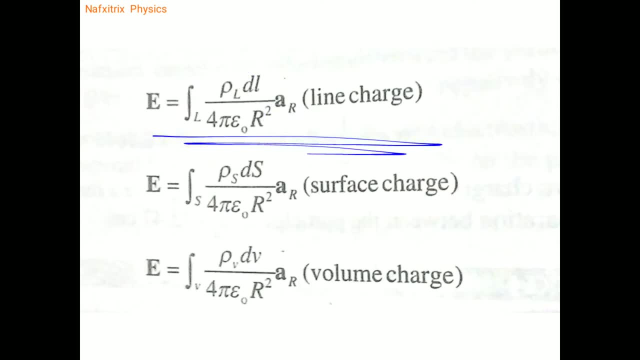 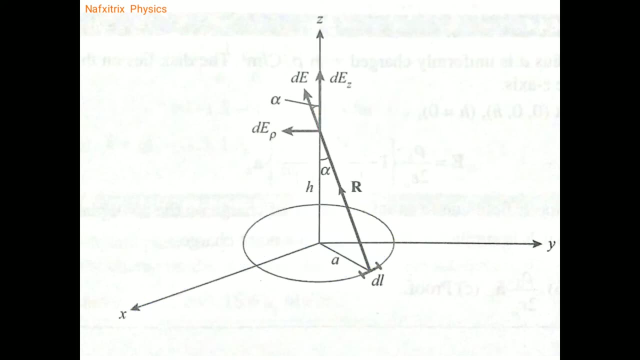 there here. so we need to use this formula for this. so first of all, this is the arrangement. so here this is the ring and here we are considering a particular element of the link dl element of the ring, not the entire ring. so we just consider a particular d element. 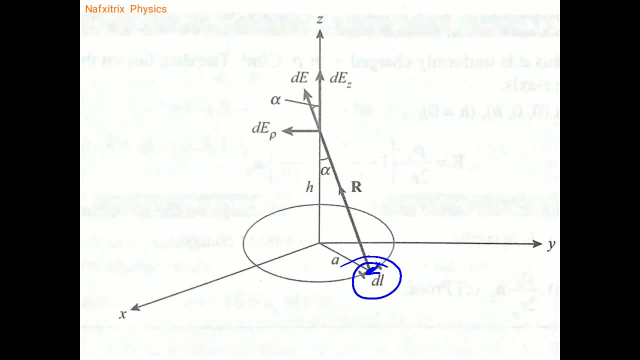 and just we integrate, because here dl is there, so we just integrate over the entire ring later on. so the we need to find it on the Z axis. so this is the Z axis. so from here to certain point on Z axis we have drawn a line. so the 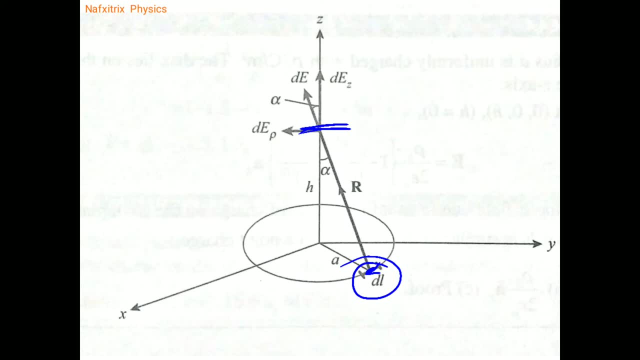 that is this, this is that line. so yes, is the ring, and it is of length R, so R, with some vector, position vector. so it is of direction, R. so that means its length and direction is R, capital R. so from here to here, the length and direction is: 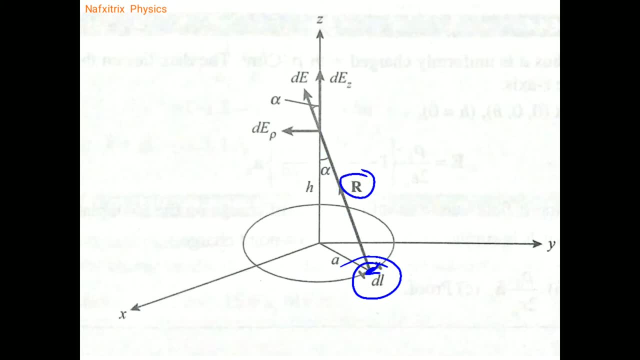 R, so magnitude is magnitude of R, and here, from here to here, electric field is acting in this direction. this is the direction of electric field. so if we consider a positive charge like that, so for positive charge electric lines of force will be acting in outward direction. so from here, because of this effect, so here it is pointing out in this direction. 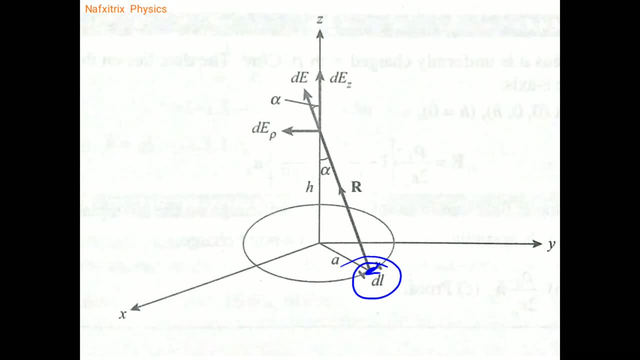 and the angle between this vector and z axis is alpha, so here also the same: the angle between d and z axis would be alpha. so if we divide that one into two components, so this is d e z and this is d e r. so this is d e z. so this is d e z and this is d e r, so d e z, d e r. so here. 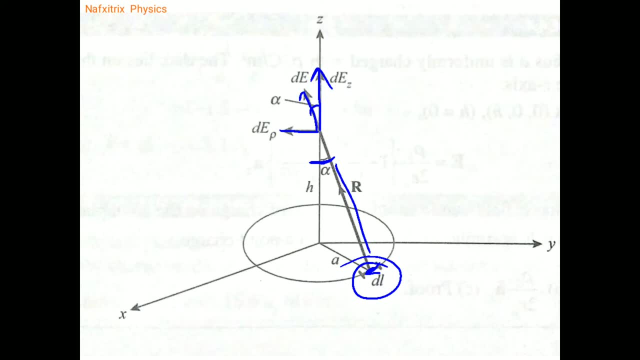 d e r, so d e r. so this is along z axis, electric field component along z axis. this is in along x y plane. so along x y plane we are having x coordinate and y coordinate, so both of them put together. here it is written as dou e rho like that, so just like r. so uh, we know that square root of x, square plus. 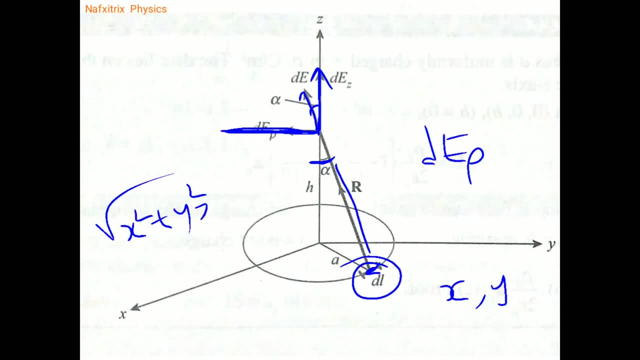 y square is nothing but r, like that, uh, y square is equal to r. so, like that, square root of x square plus y square is equal to r. so dou e r. so that is along the x? y plane, so this is so here. we should not get confused. so this is along, this is along x y plane and this is along z axis. so x? y plane. 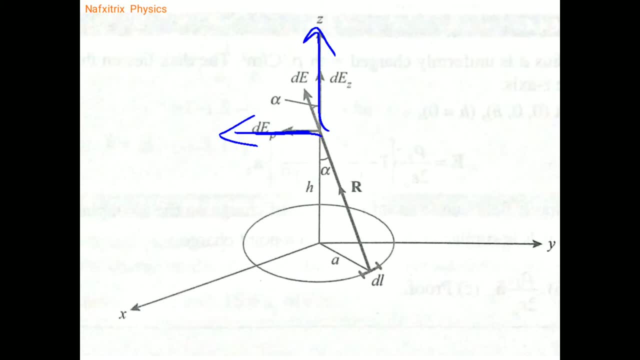 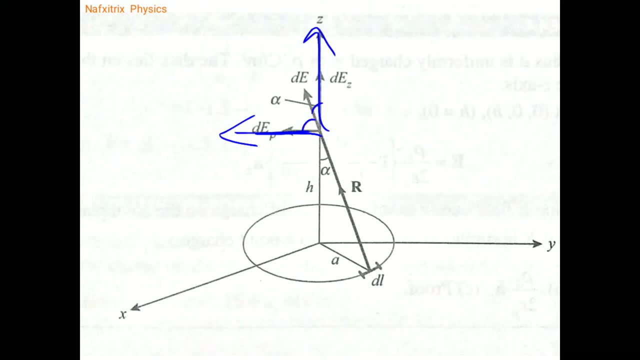 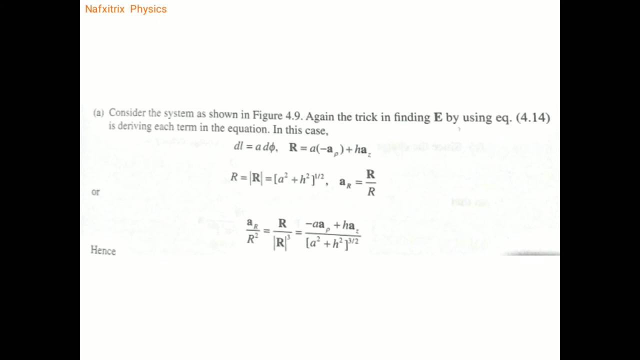 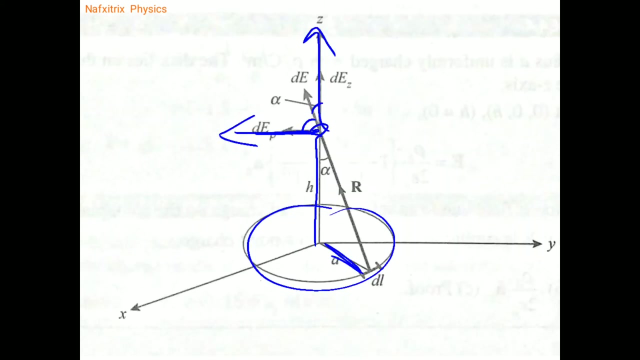 component is uh and this is z component, like that. so that is a division of component. and here, to here this from this point, the height is h and here radius of the ring is a has given. so now consider the angle: d l is nothing, but so this is some arc of length, d l. so if we define, it is making an. 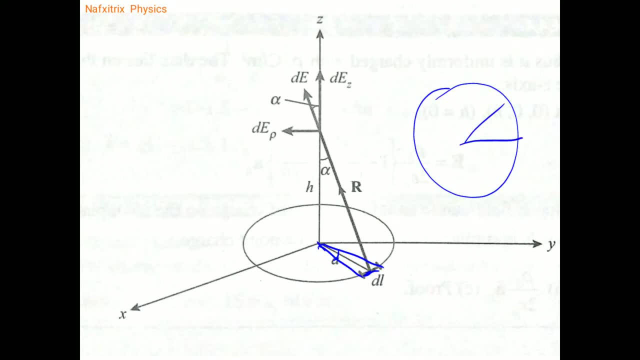 angle d five, so here. so if this is a circle, if it is an arc of length, it would be making some certain angle. theta is also, this is radius of the circle, so theta is nothing but l by r. so here in, in this case we are having d phi, so here it would be making an angle. d phi is. 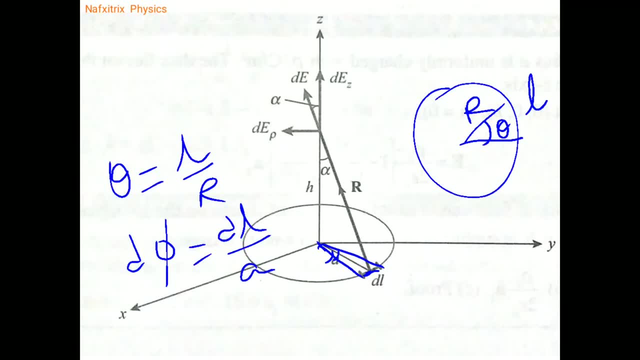 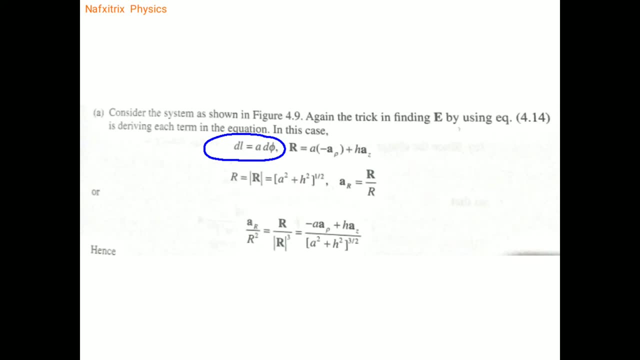 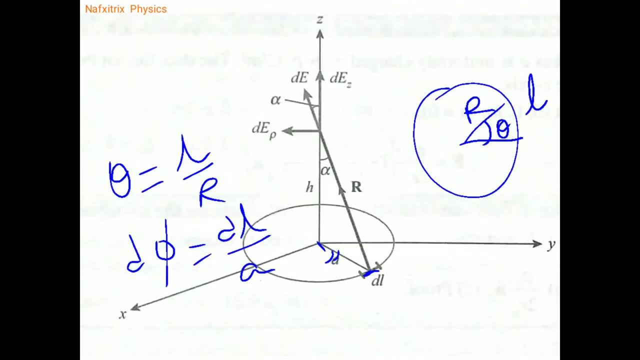 equals to d l by a, so radius of the ring is a as the radius of the ring is a. so that's why. so dl is nothing but ad5, so dl is nothing but ad5. so this is the thing we are having, and next is so this very important thing, is this one we need to keep an eye on. so this r is divided into two. 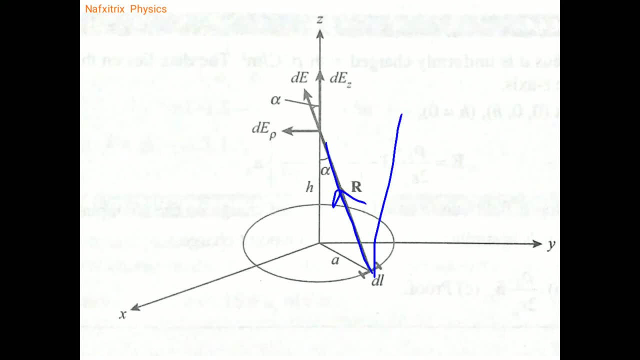 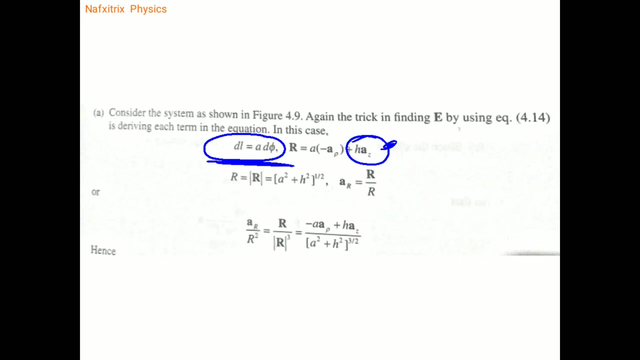 components. so one in this direction that is perpendicular to x y plane. so that is haz. so this point is at a distance h from the x? y plane. so that's why haz, az is nothing but k cap. instead of k cap here it is used as az and it is moving in this direction, from this point to in negative. 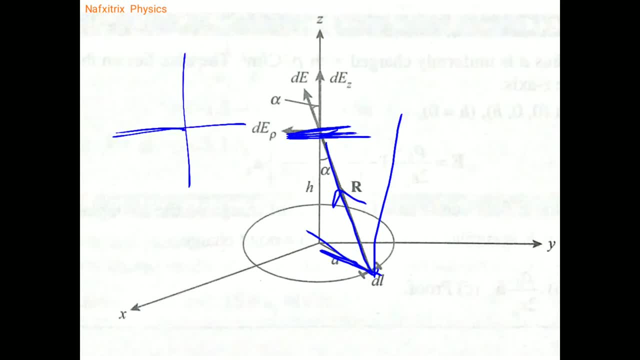 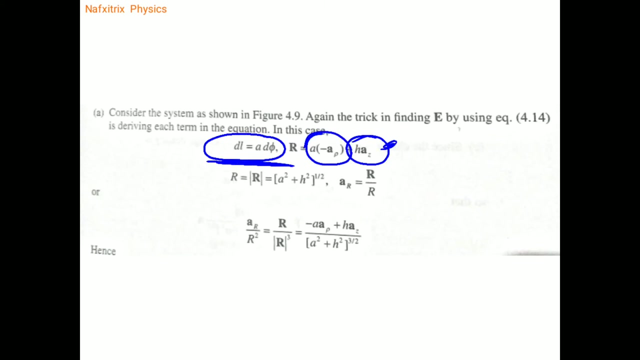 direction like that. so just like origin, this is positive, this is negative, like that we used to take. so here, here, it is not coming outwards but is going inwards, like that. so here, at this point, so that is nothing but minus k in radial direction. so so minus a rho, rho is nothing but radial direction. 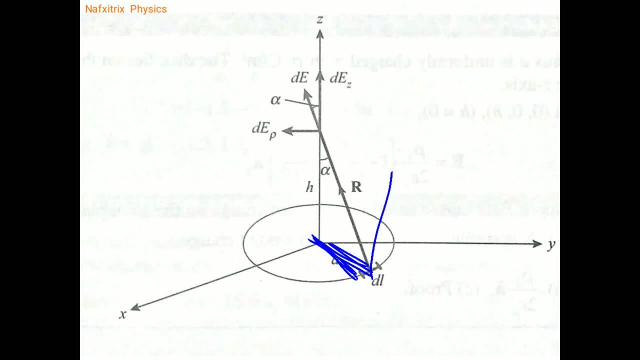 radial direction. that means nothing but x, y plane here. so here only z coordinate would be coming. so for this component only z component, for this height only z component would be coming. but for this radial direction both x and y coordinates put together would be coming. so that is nothing. 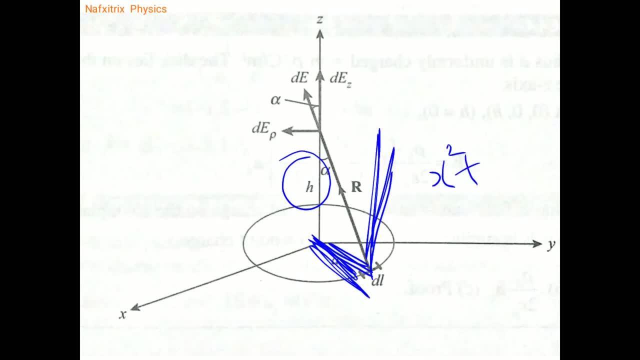 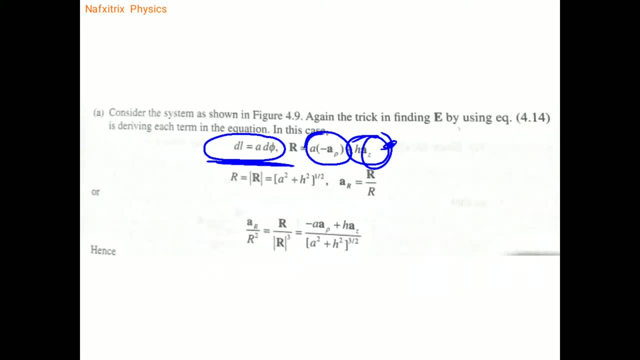 but overall it is given as: x plus x square plus y square is nothing but r square, so that is nothing but radial direction. so hence it is indicated as minus a rho. a rho is nothing but radial direction. so these are, that is about the components. so this is when we need to understand, first of all this: 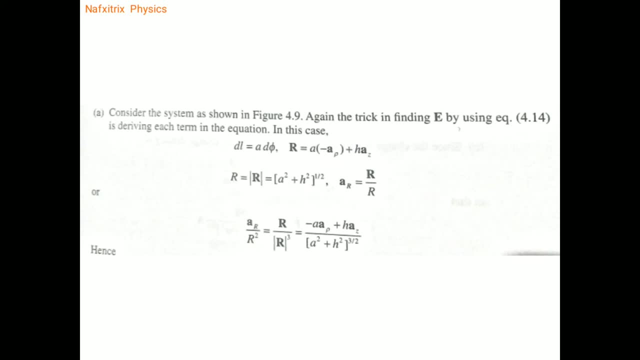 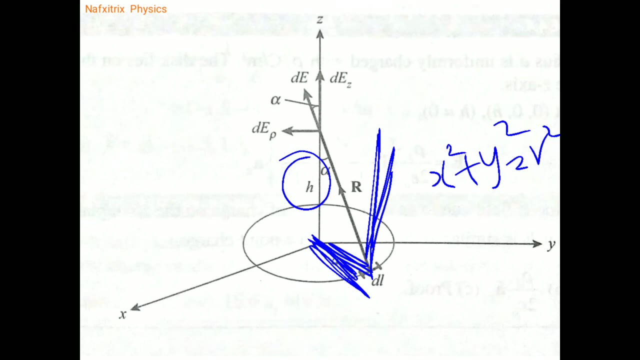 so that is how we have got. and next, magnitude of r is nothing but square root of a square plus h square. so here this is r, so its magnitude, finding its magnitude, is nothing. but this is this component plus this component, whole square. so here you can see rectangle triangle also. 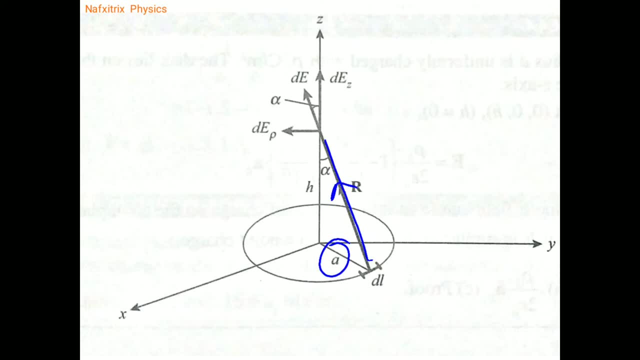 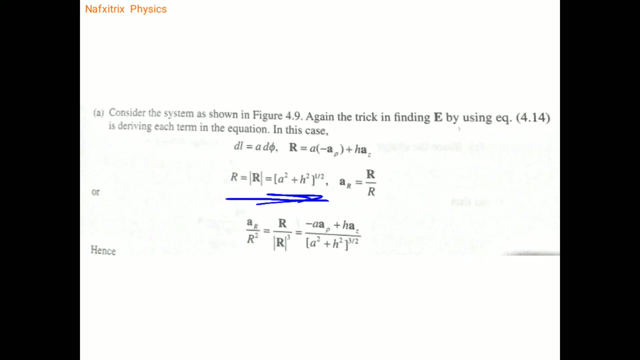 so easily. here you can see right angle triangle. so this is r, so this is h and this is a, so it is like this: h a, r, so r is nothing but square magnitude of r, the t side magnitude of r: square root of a square plus h square. so square root of a square plus h square. so we know that a r is also r vector. 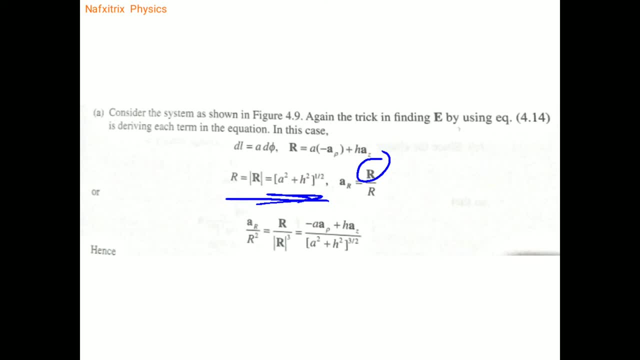 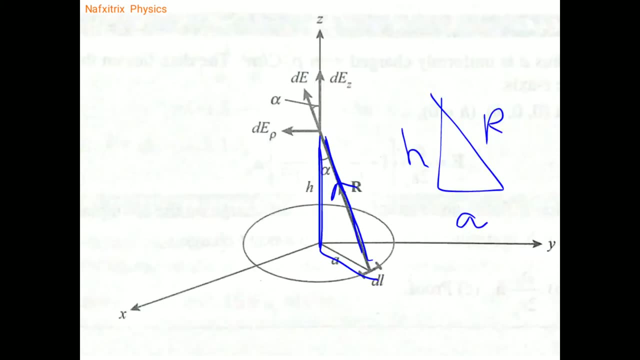 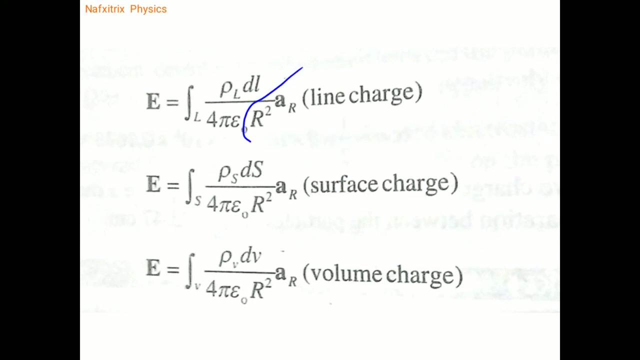 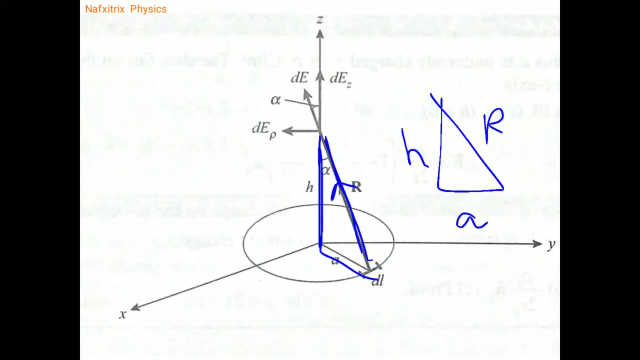 by magnitude of r. so in order to get unit vector direction. so next is we need to divide a r by r square. we are dividing because in the formula we are having a r by r square here, in the formula a r by that is unit vector in on direction, radial direction, that is, in the direction of r by r square. 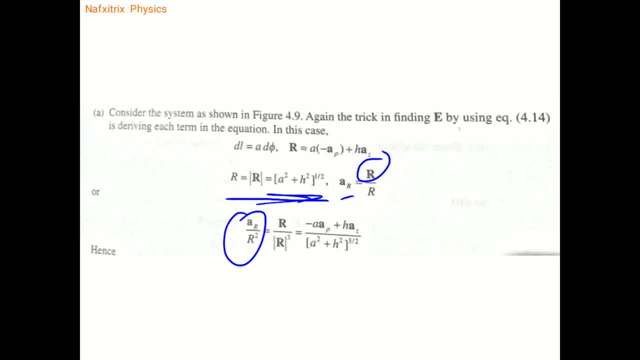 hence a r by r square. that means a r is this vector r by r divided by r square. that is nothing but vector r by r cube. so we are having r cube. so r is nothing but minus a a r plus h a z. so that one here we are having, and this whole. 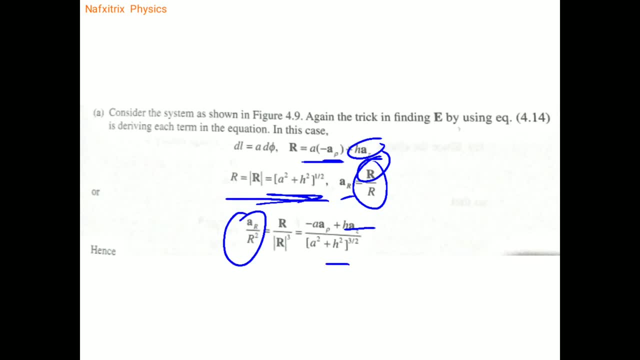 cube. a square plus h square, so r is nothing but a square plus h a z. so this is all, and we are getting A square plus h square, So r is nothing but r plus h a z, and there is a whole, and then we are getting a whole. 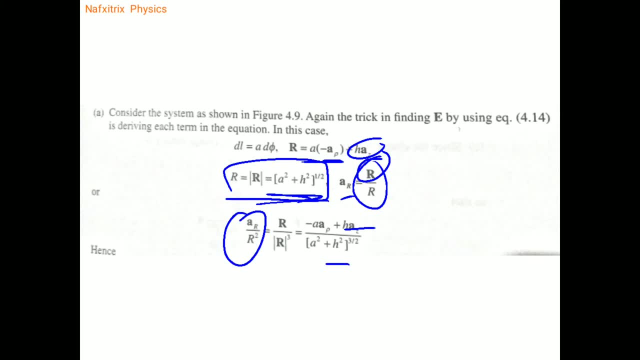 So this whole is one, that is another part of this. So all these are, So that is all the things that we are doing. okay, square root whole cube is nothing but a square plus h square whole to the power of 3 by 2. 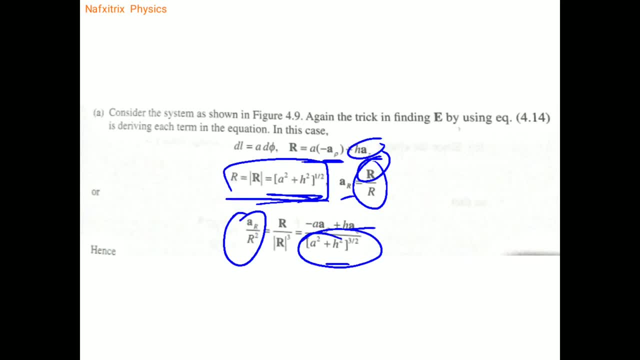 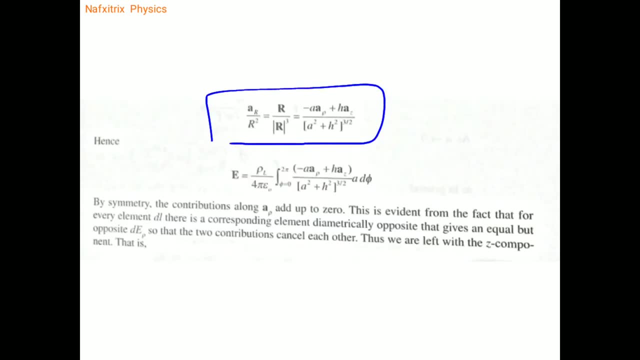 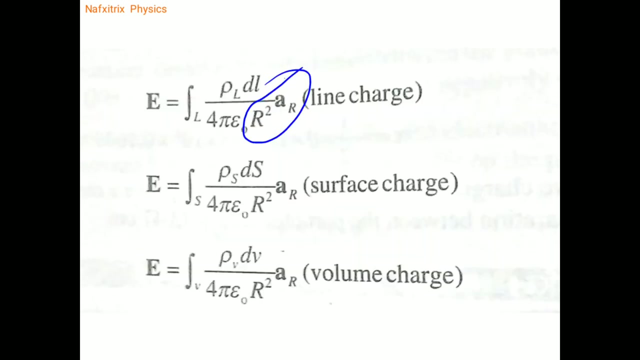 so that one we are having. so this is the thing. so a r by r square, r cube which we have derived. now, only so in the place of capital r we have placed this and r cube this. so next is we just need to place this in the formula. so formula that is in the page. so here rho l by 4 pi epsilon naught. 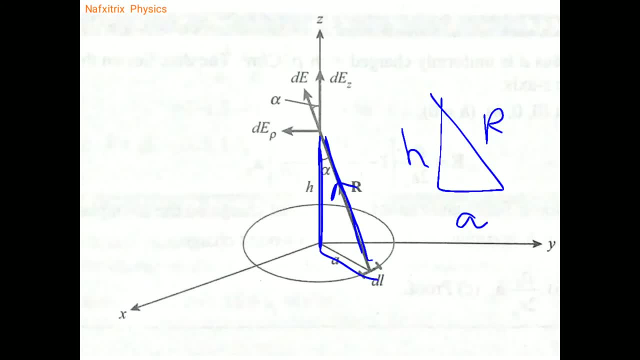 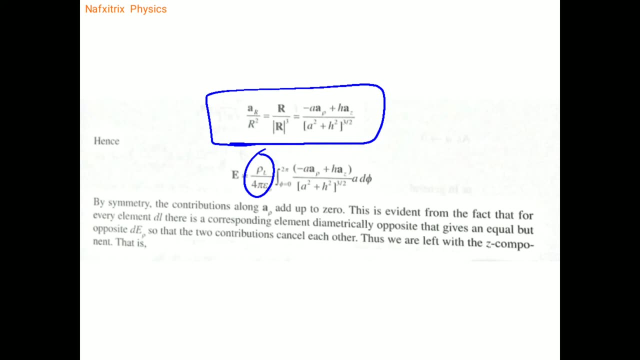 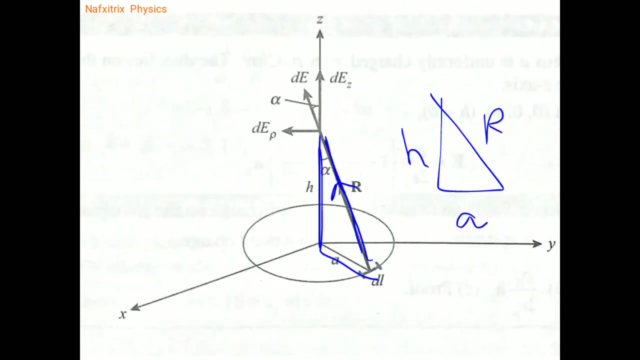 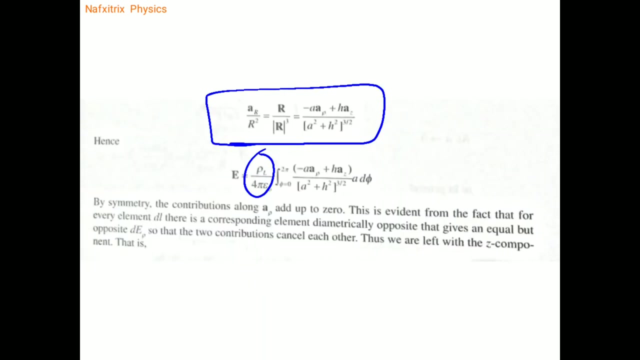 would be taken out. so rho l by epsilon naught. so rho l by 4 pi epsilon naught taken has been taken out. and and next thing is dl. dl has been replaced with this. so dl is nothing but a d phi. so it is replaced with a d phi. so a d phi. and a r by r square is replaced with this. 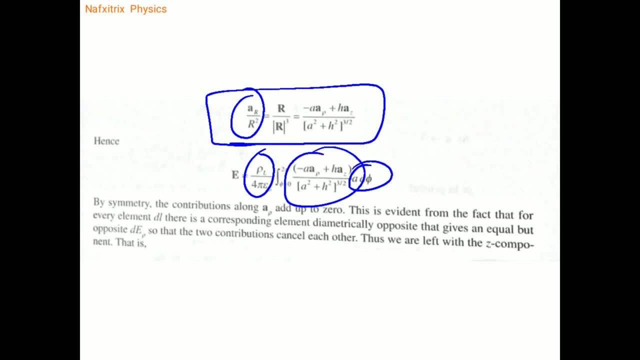 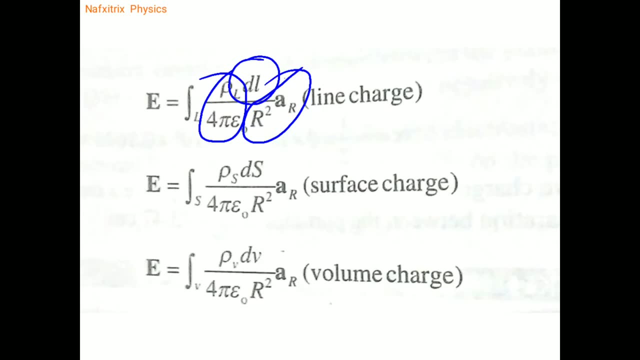 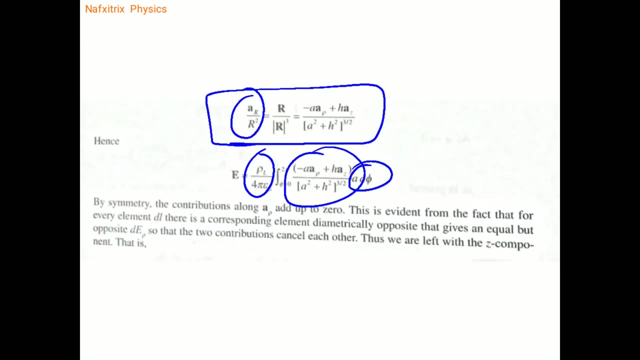 so that is the thing which was remaining. it is so. here is a r by r square. remaining thing is this only in the formula. so a r by r square. so where is it so here a r by r square is nothing but r, cube by r. so in one multiple with r and r. 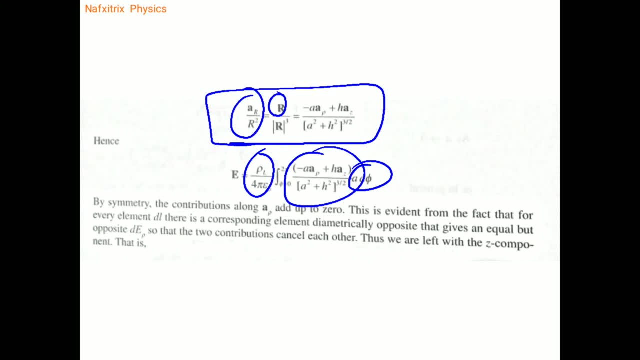 and the numerator and denominator, we will get r, magnitude of r into r is nothing but r. so this is the thing we are getting. so this is the replacement and we need to integrate from zero to pi, because we are here, d phi is there. so zero to two, five. so for the complete, 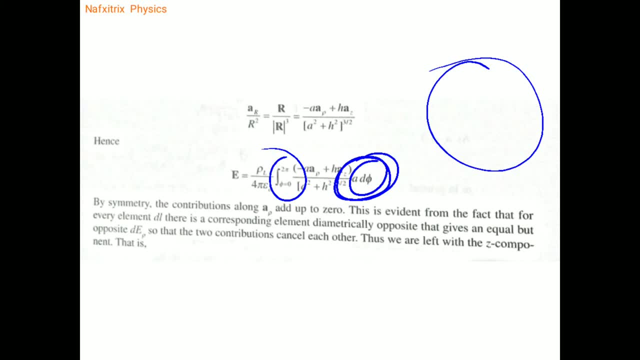 vertical zero to two. five is the angle. so now another thing is by symmetry the contributions along a or a rho add up to zero. this is evident from the fact for every element there is corresponding element diametrically opposite gives an equal but opposite. so the two contributions cancel. 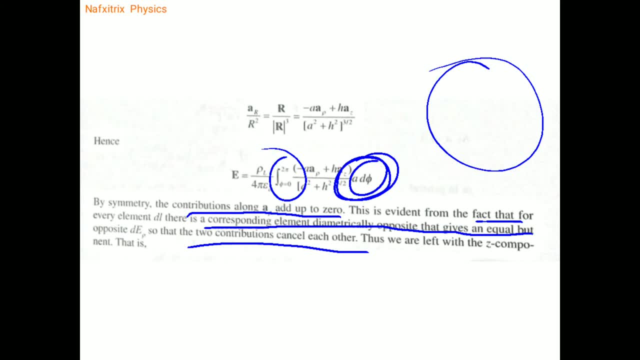 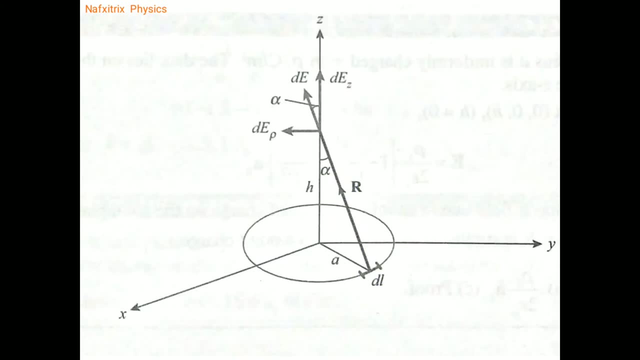 each other, we are left with z components. so if we consider the uh, if we consider this ring, so for this element, for this every element, there would be another exactly opposite element, exactly opposite to this, so it would be offering electric field magnitude in this direction. so here it would be in this direction: euro, but z component would be in this direction. 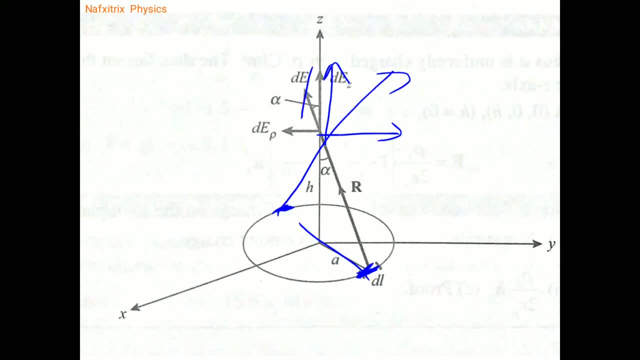 so if you see, uh, this z component, that is, this z component and this z component. both are upward direction, but this ar component and this ar component would be in exactly opposite direction and of equal magnitude because of the symmetry- symmetry in distance, symmetric circle. so they both would get cancelled, only z components would be remaining. so it is just like. 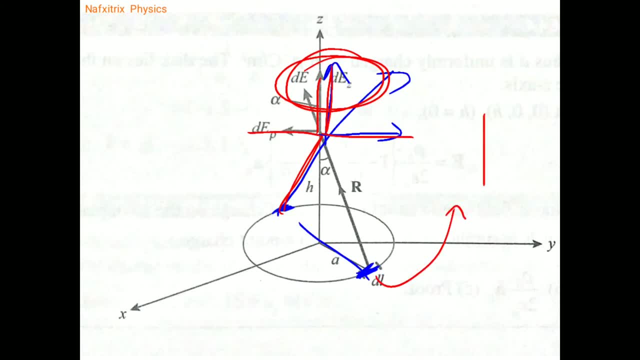 for the for this element, ez is in this direction, ez and e rho is in this direction. and for this component, e rho is in this direction and ez is in upper direction only. so these both directions, that is, these both directions would get cancelled up, only these directions would be remaining, so they both would add up. so we can neglect radial components in. 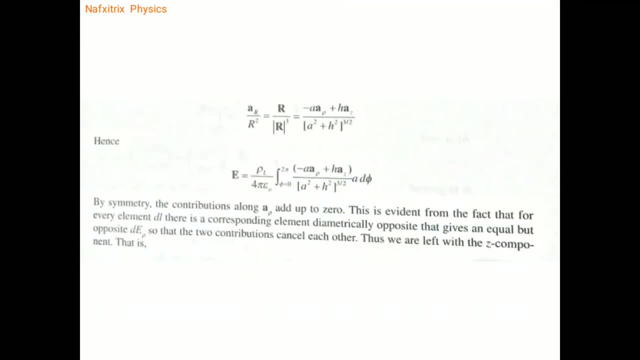 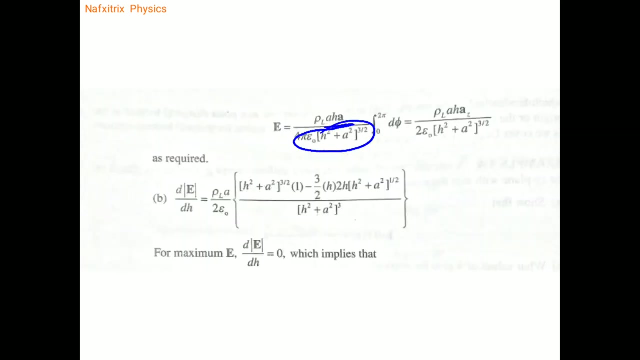 formula. so that means we can neglect this component. a rho, you a minus a rho. so only what would remain is haz and this entire thing. so hence here, haz and this entire thing: h square plus a square whole to the power of 3 by 2. only that one is remaining. 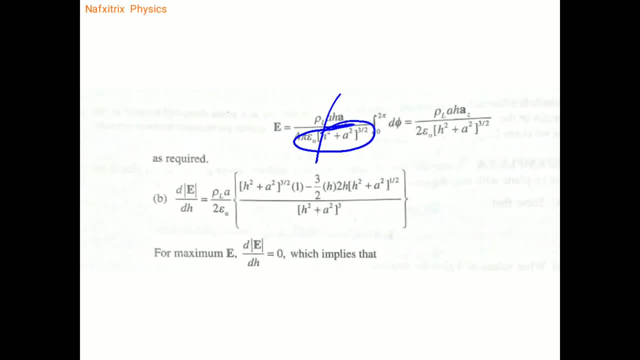 and 0 to 2, 5 d 5. so 0 to 2, 5 d 5, and here a has been taken out, so a has been taken out. so this is the thing we are having. so this would be remaining and we need to integrate. 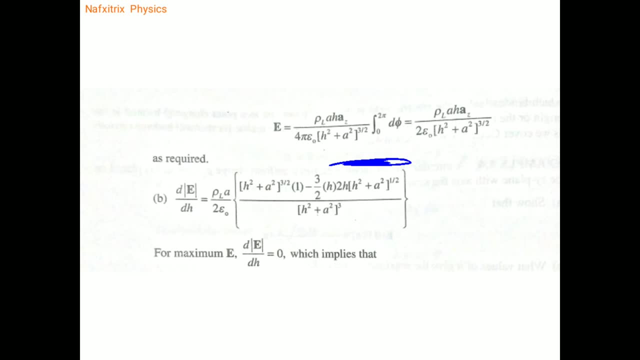 it from 0 to 2 pi. so integration of d: 5 is nothing but 5, the 5: 0 to pi, so 2 pi minus 0. so getting 2 pi and pi pi would give cancer to 1, 0 to 2, 0, so 2 epsilon naught. 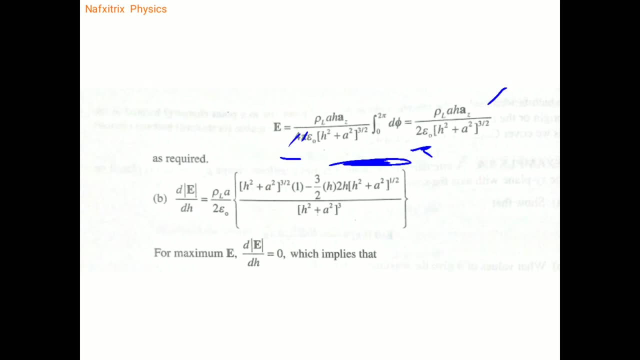 so rho, l, a, h, a, z, cap and h square plus a square whole to the power of 3 by 2. so this is the remnant, so this is the thing which was asked. so finally, we have found electric field because of the circular ring whole to the power of 3 by 2. this was asked, so it is. 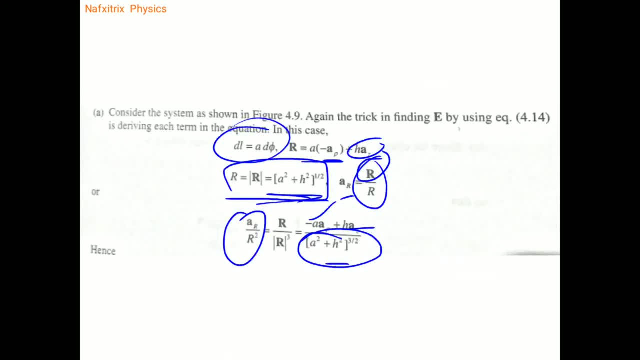 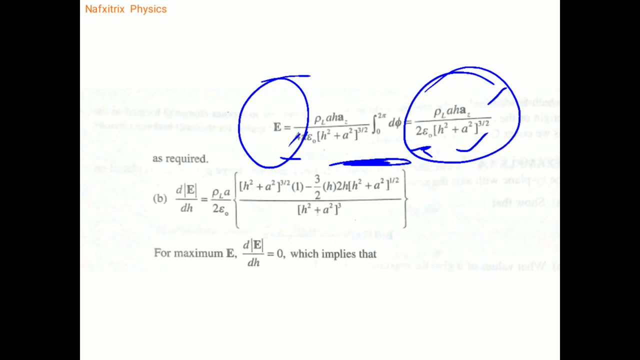 same as this, which we have proved now. so next thing, so next thing, and next thing is: they have asked us at what value of z e would be maximum. which value of z e would be maximum? so z is nothing but h, with height, how the electric field is varying. 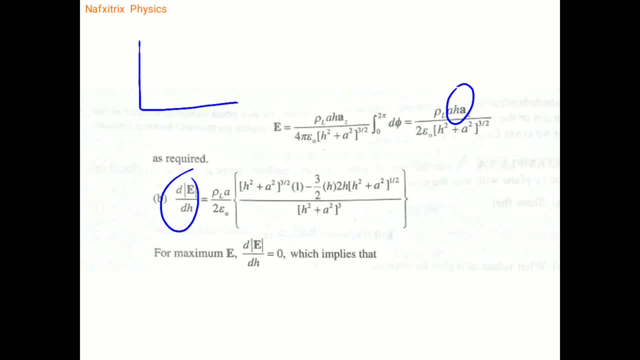 so if dou e by dou z, so if we suppose, if we draw a graph between e and h, so e and h, so suppose it would be like this: so at some particular point electric field is varying, to some particular point electric field is magnitude, if we draw it aniden, so here tangent. 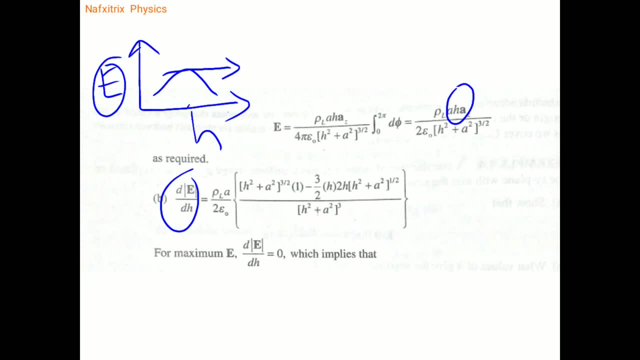 is nothing but dy by d x, so de by d h, so that must be parallel to this. hx. that is nothing but tana slope is nothing but tan theta tan. 0 is 0, so parallel to this axis, h axis. so hence, d, Ted b, Fam Veronica must be equal to 0, so the PD has be equal to 0, so hence, we are differentiating this with respect to H. so on differentiatinglles, we have tomorrow's computer as well. so that is that over here is周ors into C, q, potassium. so now let's think about creative Plan: H by D, X by L to be 0, and here heading towards C, p revenue. 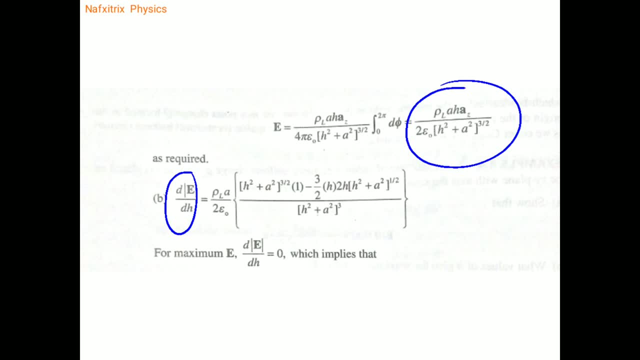 of flow rate is power. that is equal to omega to K. T is equal to minus E, equal to Islamic value minus E by購, which is the general deviation. then let's see at the desktop we have given differentiating. so here in the numerator also we are having h. in the numerator 1h we are having 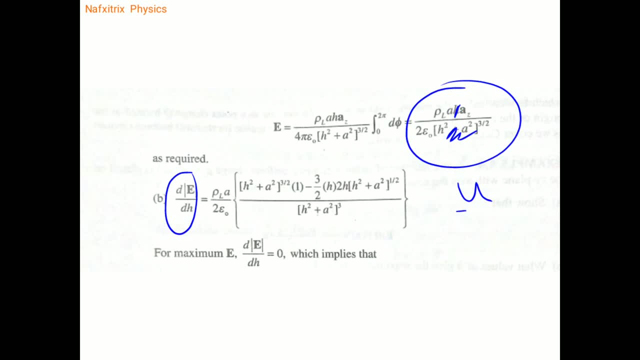 and here also h function is there, so it is just like u by v. so we need to use the formula v du minus u, dv by v, square on differentiating this term. so here rho l by 2 epsilon naught, rho l? a by 2 epsilon naught is there. so rho l? a by 2 epsilon naught, like that, so v as a square plus a. 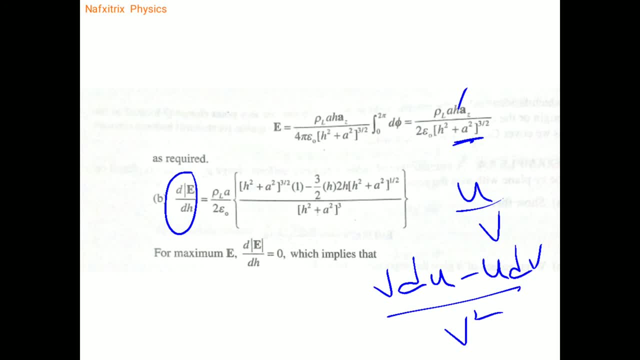 square, whole the power of du. so dh by dh 1 minus u dv, minus this u dv, u is nothing but here h. so in the place of u we are having h here in the place of v. h square plus h square by 2. epsilon naught is there. so rho, l a by 2, epsilon naught is there. 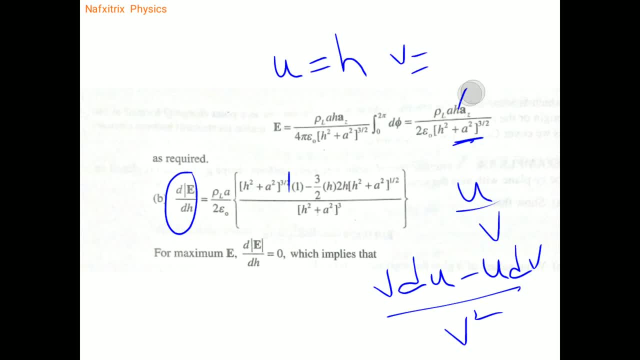 plus a square whole to the power of 3 by 2. that is this entire thing. h square plus a square whole to the power of 3 by 2 is there in the place of this. so v, du minus u, dv, u is nothing but h. 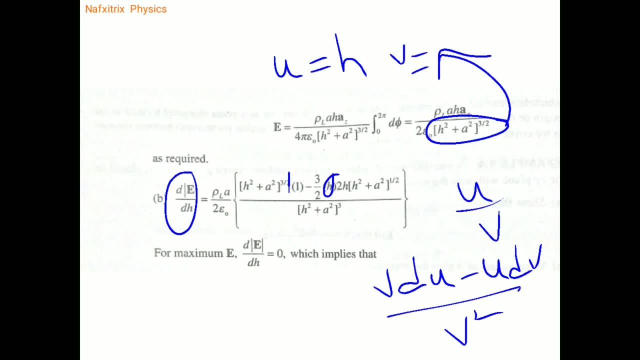 and differentiating v. uh, we were n into x power, n minus 1. so 3 by 2 into h square plus a square whole to the power of 3 by 2 minus 1. so that is nothing but um a half square root of half. 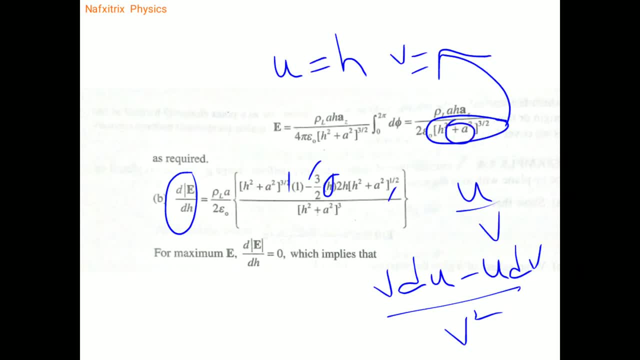 and again we need to differentiate this term, this function, so on, again, differentiating 2h. so we are getting into 2h. so that is the thing. so if we differentiate this v value, we would get this entire thing except h. so this is based on the integration. 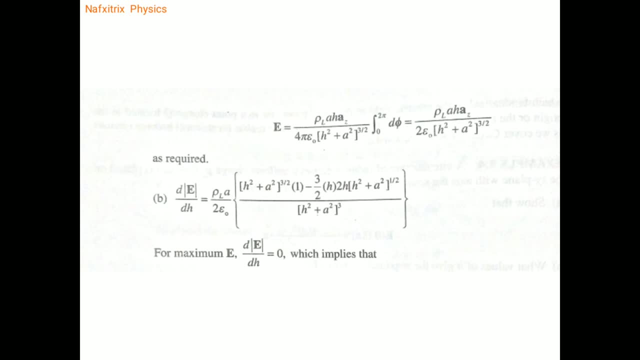 and next thing is: so it is based on the integration h square plus a square whole to the power of 3 by 2, um, so on, sorry, it is based on differentiation. so, on doing differentiation, we will get, and finally, uh, by v square. so v square is nothing but this whole square. that means 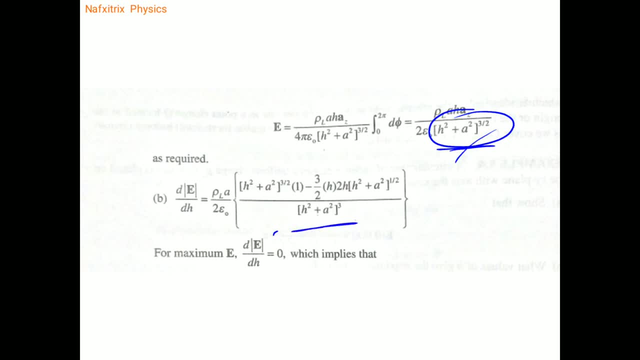 3 by 2, whole square 2. 2 would get cancelled, whole cube. so h square plus a square whole to the power of 3.. so for e to be maximum, d, e by d, h must be equal to zero. so this entire thing must be equal. 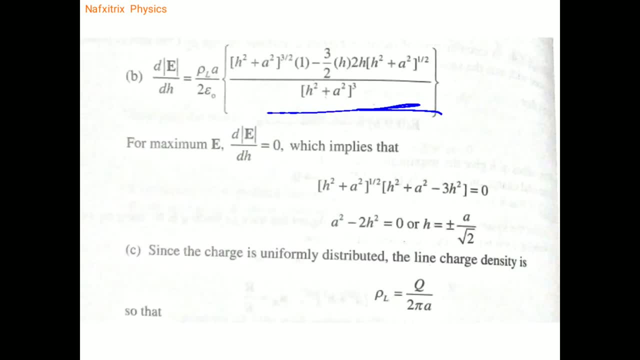 to 0, so this thing must be equal to 0. so this, everything would get, this, everything would get: uh, go to that side and what would remain is only this thing: the numerator value. the value of the numerator would be remaining. so here we need to just take a square root of h square plus a square out. 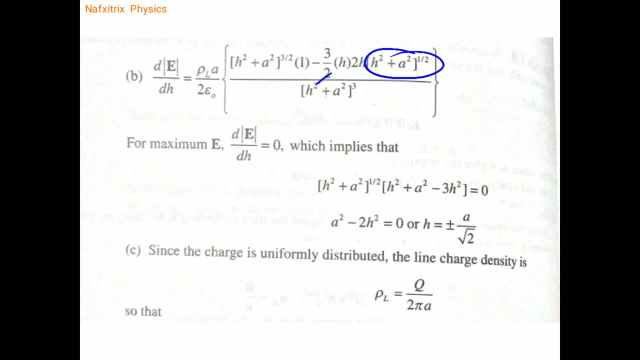 so from here what would remain is 2- 2 would get cancelled- minus 3 h square. so minus 3 h square and the square root of h square plus a square. here also, uh, h square plus a square would be remaining here, square root of a square, h square plus a square, if you, if we take comma h square. 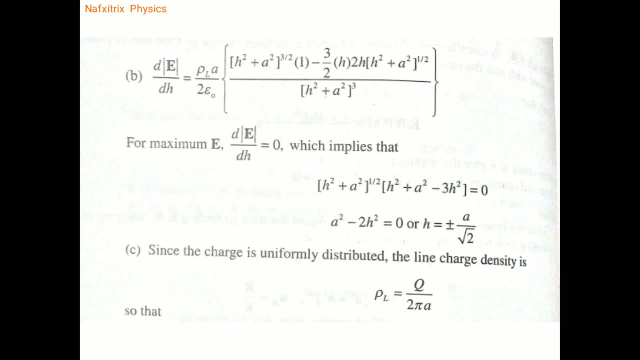 plus a square would be remaining, so that h square plus a square, and- and this we just need to equal it here- does that make sense? 0? so here, if we do equate this, so here, if we see um a square minus uh, plus h square, minus 3 h square, that is, minus 2 h square. 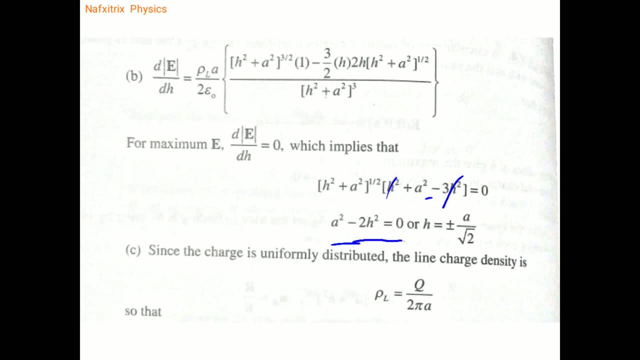 so a square minus 2 h square equal to 0. so sending the 2 h square to that side, so 2 h square, so a square is goes to 2 h square. i'm taking- sorry, i'm taking- square root, uh. so sending this 2 to that side, a square by 2, that is a by root 2 plus or minus a by root 2. so 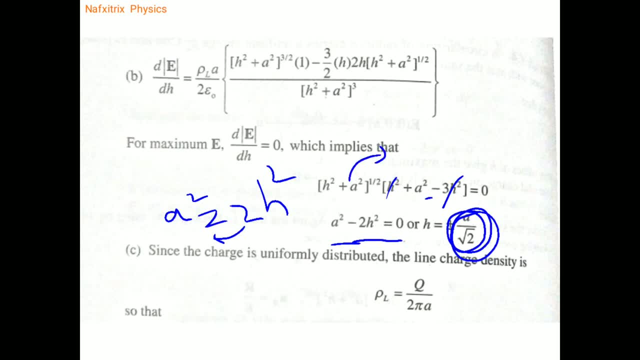 that is the thing we are getting. if we equate it to 0, we would get, in negative terms, minus. i like that because h square is goes to minus a square like that. so minus i like that we will get. so we don't want complex numbers. so h is nothing but plus or minus a by root 2, so had this height. 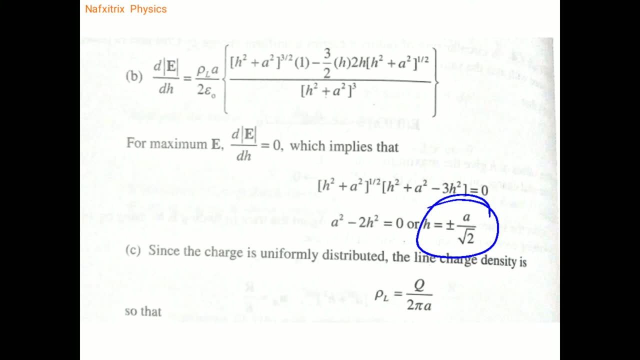 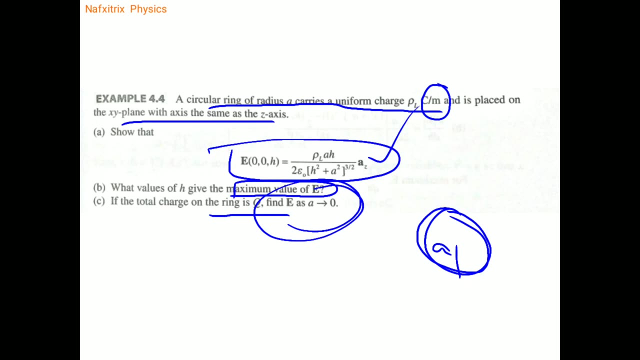 a by root 2 height electric field would be maximum. it's based on this and next what they are, as the is in the question. so, uh, next, what we need to prove is if the total charge on the ring is q, find e has a tends to 0. so the total charge on the ring is q has a tends to 0. that means if the 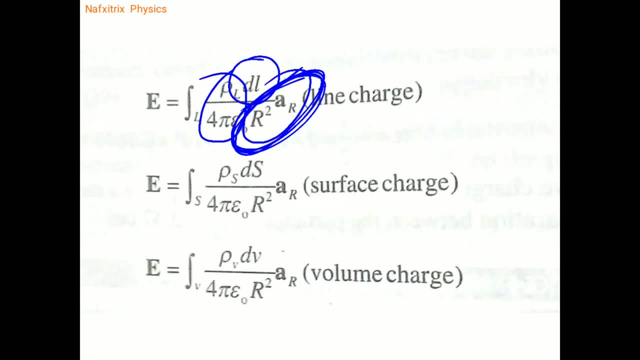 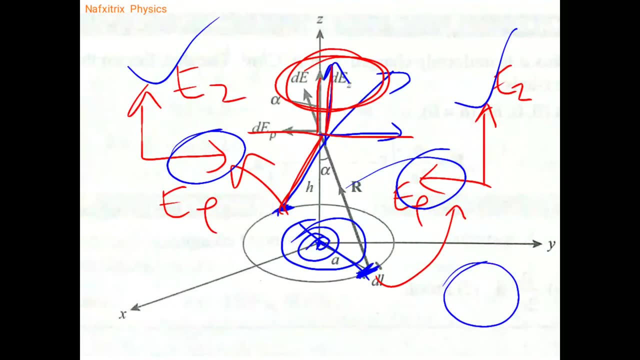 radius of the ring tends to 0. that means, if this string goes on shrinking, shrinking, shrinking and finally if its radius becomes 0, the ring is going on shrinking, shrinking, shrinking and is getting concentrated to a certain point. so the entire ring is having charge. capital q. 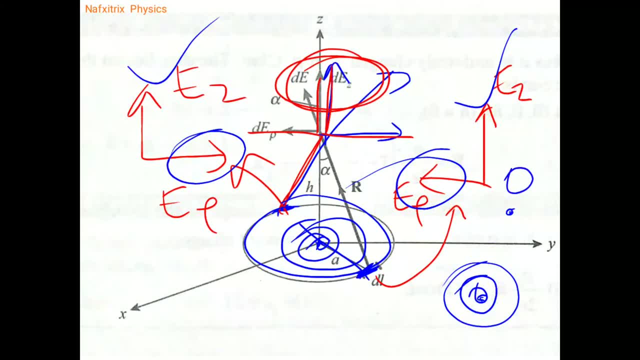 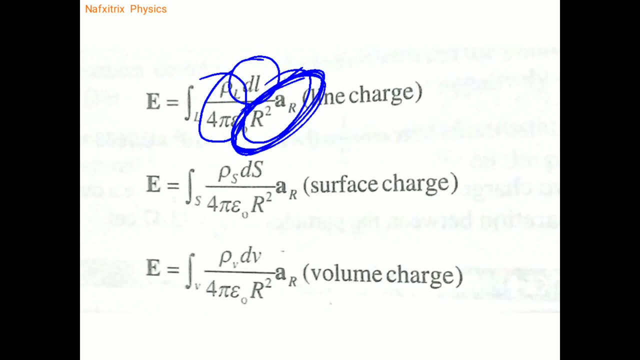 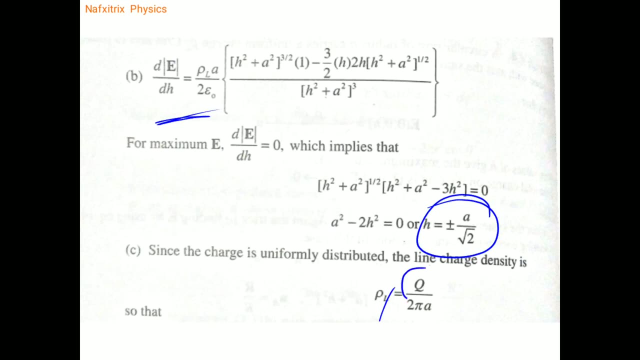 if it shrinks, finally it becomes a point charge q. so at that time what is the electric field that one? they are asking so for that. so we know that uh, charge per unit length is nothing but q. the entire ring is having charge q and its length is 2 pi r because it is a ring circle. 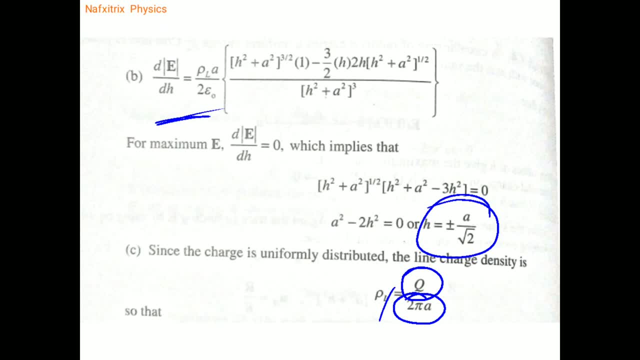 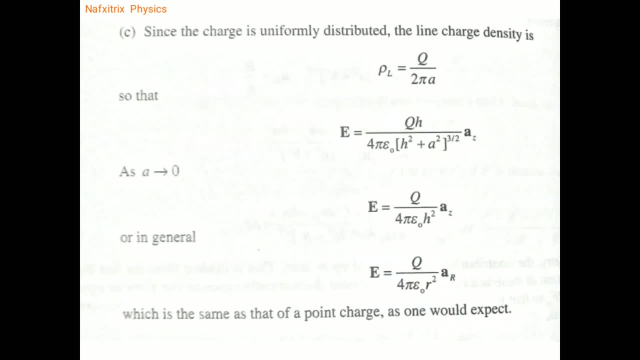 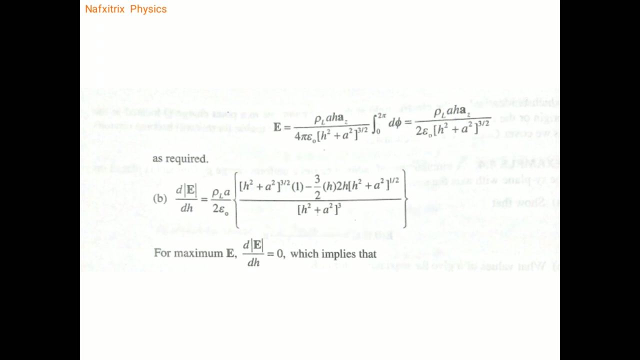 r1, so length of the ring is nothing but circumference of the ring. so 2 pi r, 2 pi a. a is the radius, so q by 2 pi a. so we just need to substitute this in electric field formula. so here this is the electric field formula. so in the place of royal uh, q by 2 pi a. 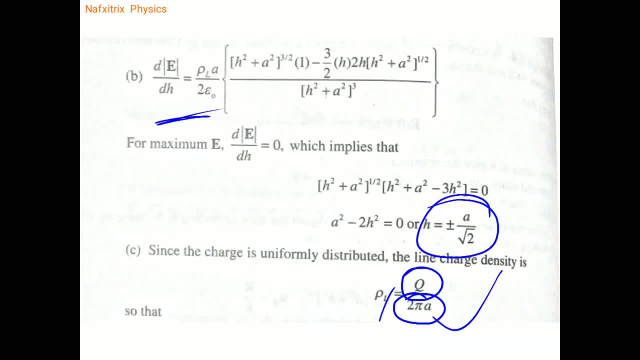 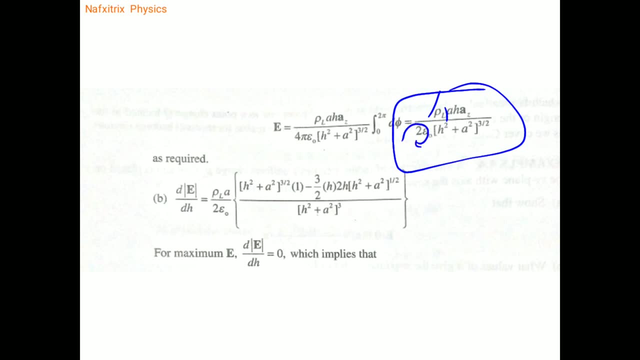 so q by 2 pi a would get cancelled, so here already 1a is there. so in the denominator 1a 2 pi 2 into 2, 4 pi epsilon naught would become, so from there we have got so 4 pi epsilon. 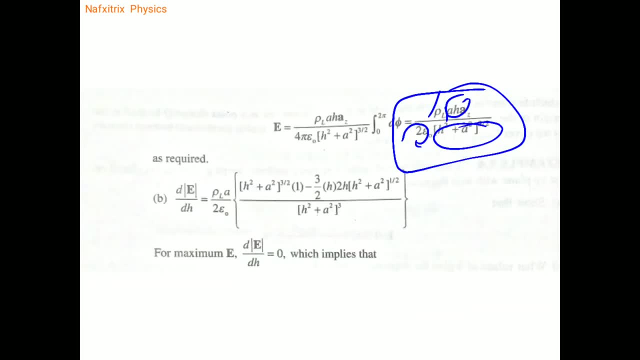 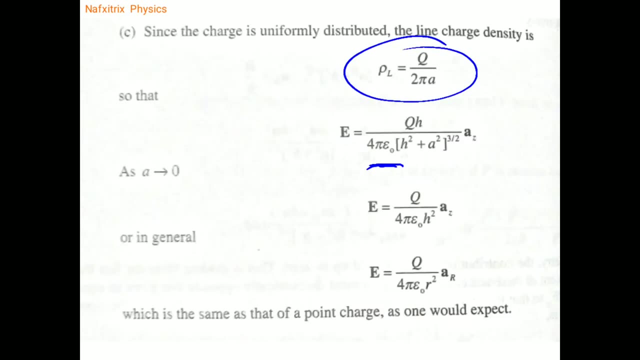 naught and H, and this entire thing would remain as usual. a, a would have get cancelled. so finally you would have this: a, z and here, as a is tending to 0, so a tends to 0 they have given. so in the place of a we need to keep 0 H square. 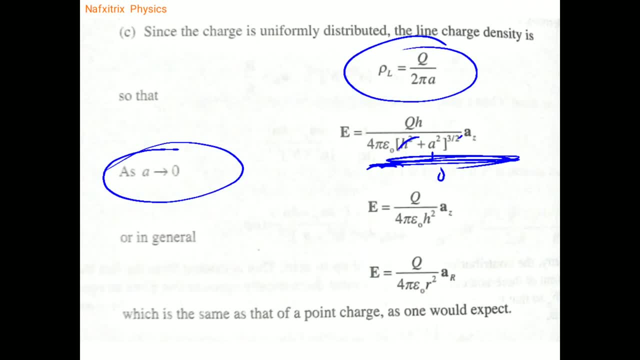 whole over 3 by 2. so square square would get cancelled and H cube- that is number H cube we are having H and 3 would get cancelled. H square Q by H, square Q by 4. pi epsilon naught H square a, z. so in general in the place of H we could 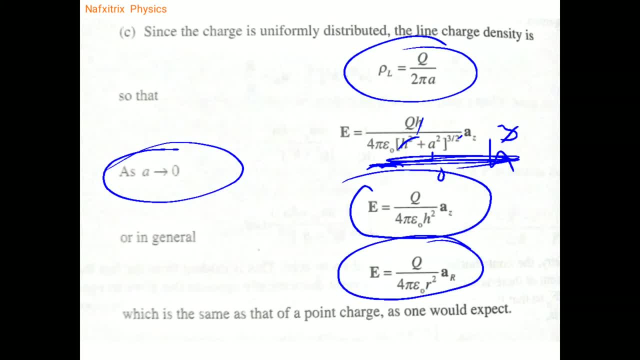 replace it with R square. so Q by 4 pi epsilon naught R square a R, so this is same as that of the point child has. one would accept. so for the point child 1 by 4 pi epsilon naught Q by R square. now that is the 1 by 4 pi epsilon naught Q by R square. 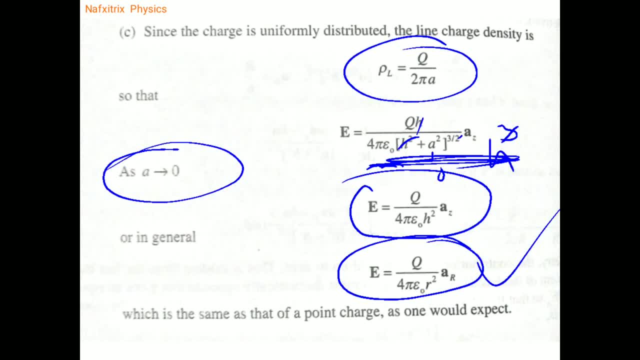 that is the value of electric field, so the same value we have got. so after simplification here, a square has been eradicated, so a is nothing but zero. so it has been eradicated. 2, 2 would get cancelled and H cube, H, H would get. 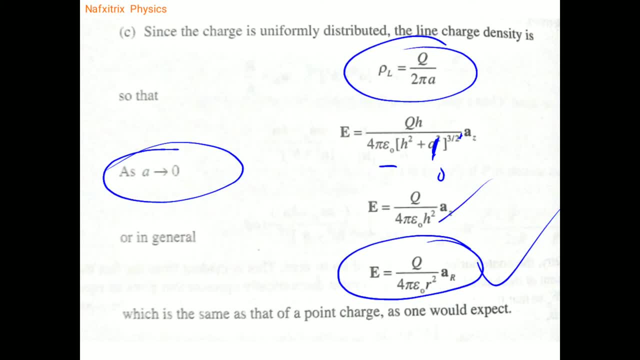 cancelled. so Q by H square, so Q by 4 pi. epsilon naught R square AR. so same has for the point charge. we will get so same thing we have got from this derivation. so finally it is correct. so this is the solution. these are the problems side by.